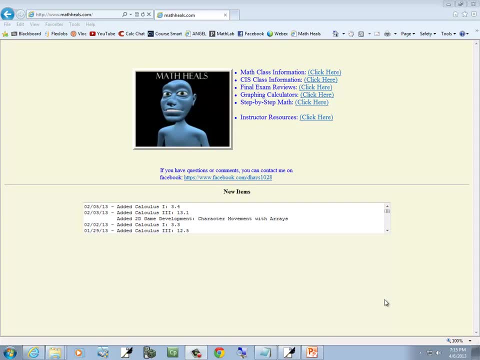 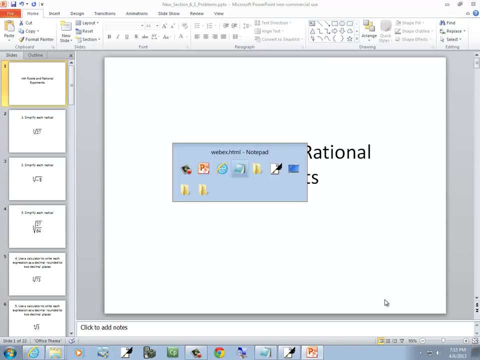 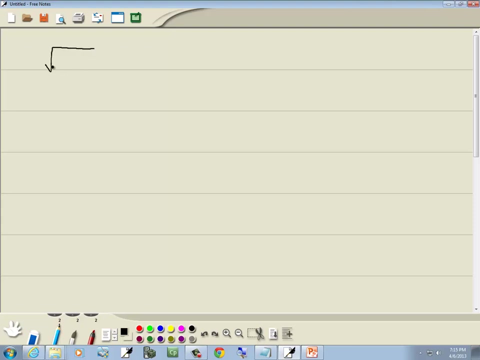 This is mathhealscom, where you can find more links to math and computer science YouTube videos. Let's take a look at int, roots and rational exponents. Now, this is a radical right here. It looks something similar to that And you've got something underneath. 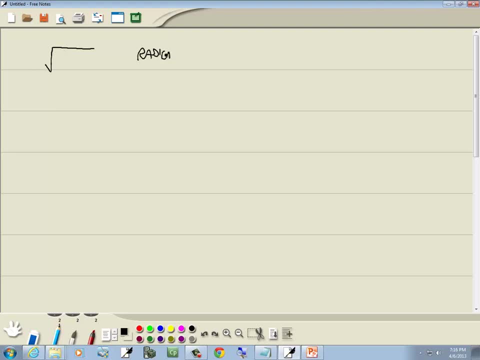 um, radical. now, some of them may look like this, where you have a number in this little slot right here. that's called your index. now, uh, this is referred to as the cube root. this one would be the fourth root. that's why they say int root. 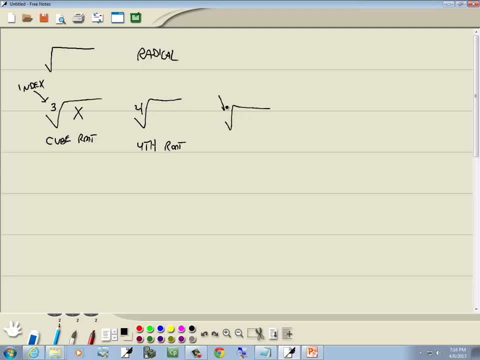 now, if you have just this symbol here and there is no number, by default your index is equal to two. this is called a square root. now we're going to explore um in more detail what the index means, with examples. uh, but those. that's our beginning. 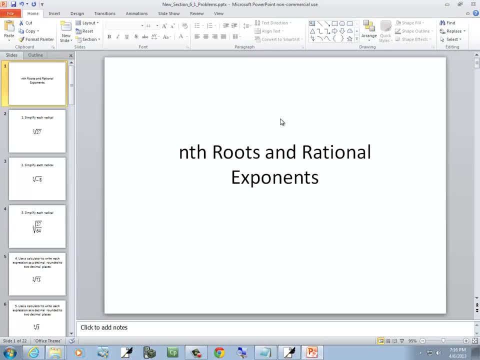 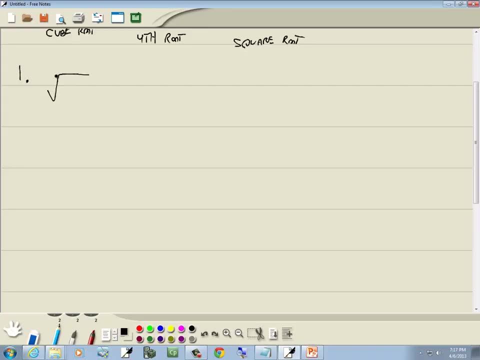 beginning definitions and let's take a look at our first problem. Here's our first problem. we want to simplify the cube root of twenty-seven. Well, we need to do the prime factorization of the number that's inside a radical. Twenty seven is three times three times three. now our index is numbered as a slot. here is three. 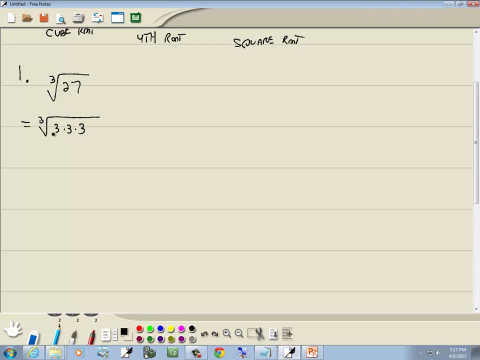 what that means is we're looking for a set of three of something. well, here we have three threes, so the three threes are going to come out in front of us, front of a radical, as a single three. so again, the index tells us how many we're. 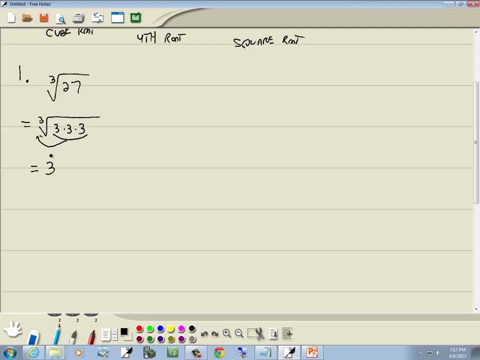 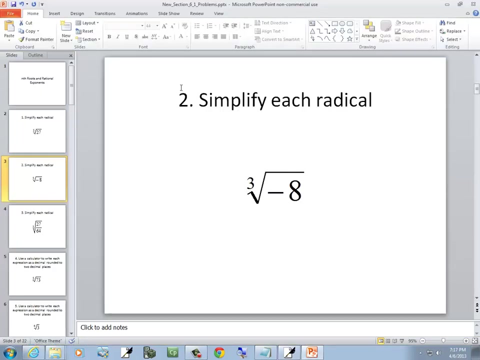 looking for and then, after you find that many, you bring it out and it comes out as a single one of them, and that's our answer. this one has a note that goes along with it that I'll talk about after we work. the problem now, our index- is. 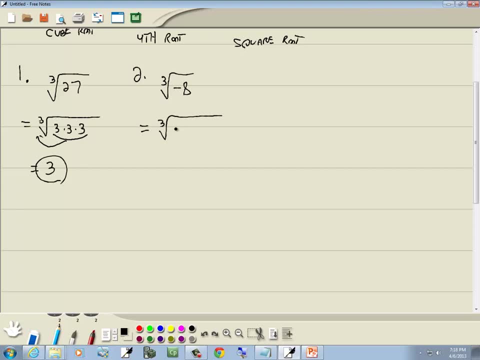 three, which means rolling for a set of three of something. but negative eight we can rewrite as negative two times negative, two times negative two. now I've been really vague there. I said: a set of three of something doesn't say what it can be, it can be anything. well, here we have three negative twos, so those three. 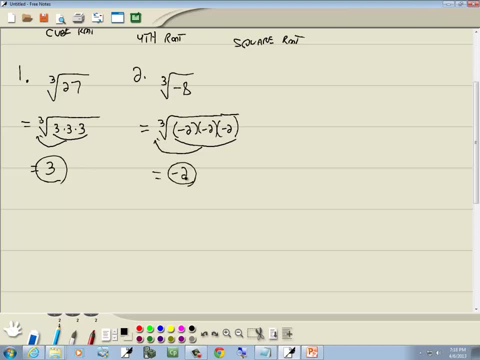 negative two is going to come out in front as a single negative two. now our note on this says if you have an odd index and a negative inside the radical, so and a negative inside the radical, you can just take. you can just take the negative out in front. 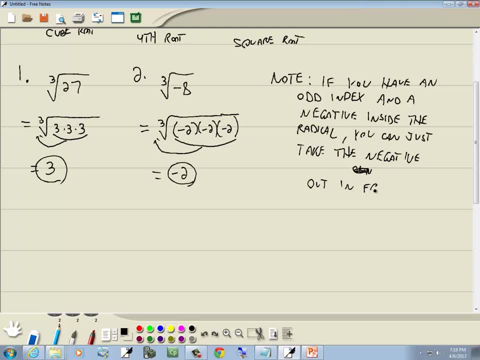 oops out in front. so for that example, there I started out with a cube root of negative eight. that says if you have an odd index- which we do, three- and a negative inside the radical- we do- it's right. here you just take negative and out in front. so just to begin with, we just 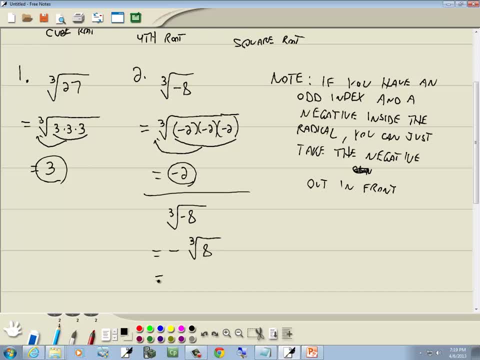 immediately put the negative out in front and not worry about it. that makes it a lot easier in problems. you don't have to worry about that. then we work in the same way. we try to come up with something. times itself, three times, it gives you, gives you a. well, the prime factorization of eight. so we got two. 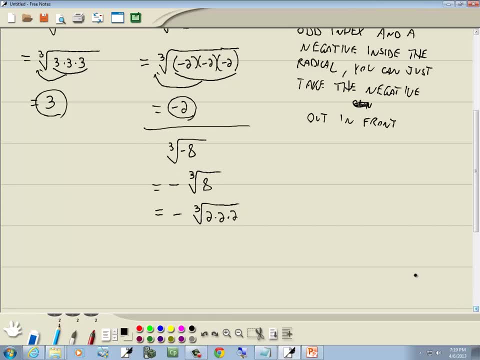 times two, times two. specifically in this section, everything will come out perfectly, I was getting ready to say, but in general, as we get into the other lessons, you'll find that not all the time will be radical, disappear. but our index is three. we're looking for a set of three, something here's three, twos, so 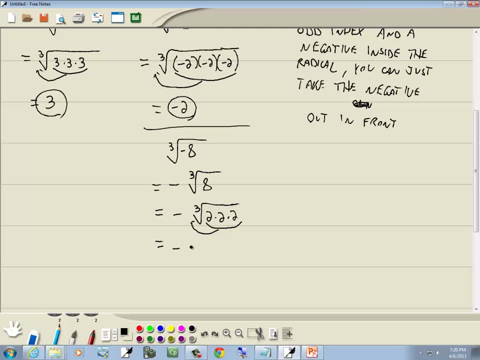 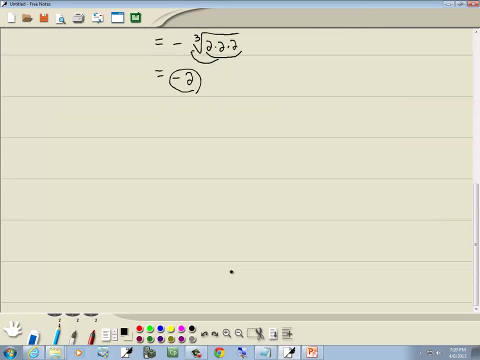 three. twos gonna come out in front as a single two. now, negative is already there and we just bring out a single two, so our answer is negative two. yeah, let's take look at the next problem. we've got the cube root of 27 over 64. well, I'm. 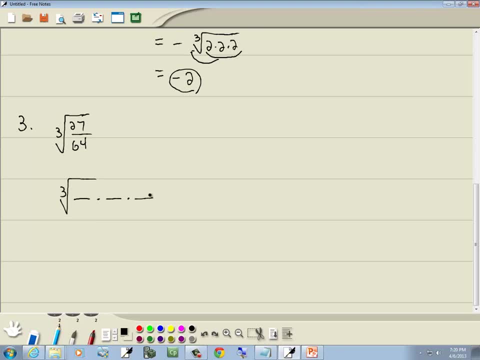 looking for set of three of something, and this one is designed to work. come on nice, 27 is 3 times 3 times 3 and 64 is 4 times 4 times 3, so our answer is negative: 3 times 3- and we're looking for a set of. 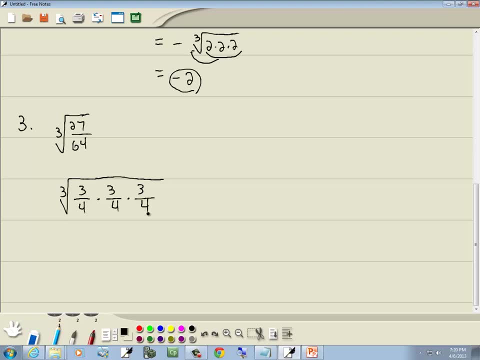 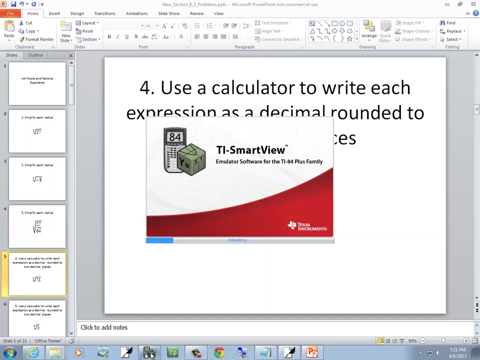 times four times four. well, our index is three. we're looking for a set of three, of something. here's three, uh, three-fourths, so we're going to come out in front as a single three-fourths and that's our answer. now the next ones are calculator based, so let me bring up my calculator. 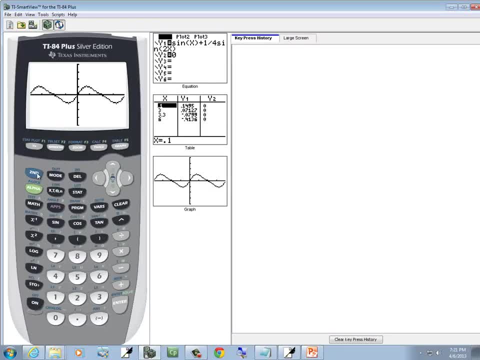 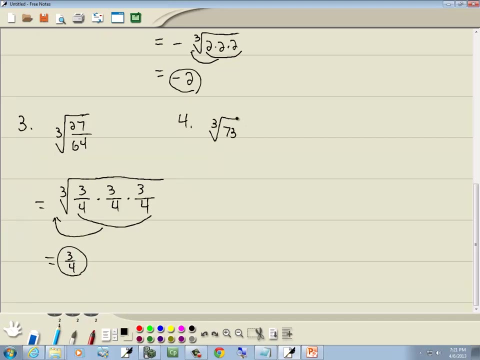 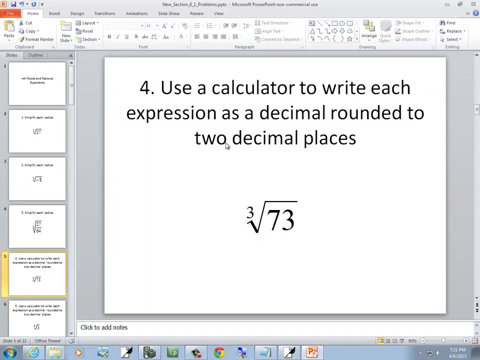 okay, we got the cube root of seventy three. well, i'm guessing seventy three's prime. i can't think of any way to break that down. uh, so to do that on our calculator. if i can get to the calculator, we're going to press our math button. 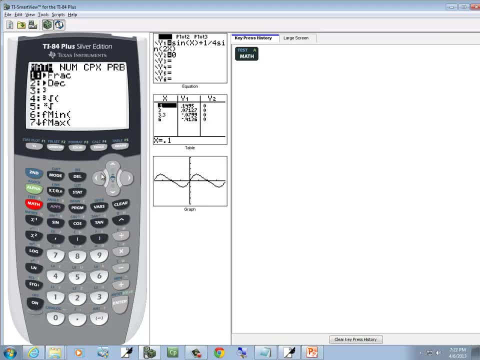 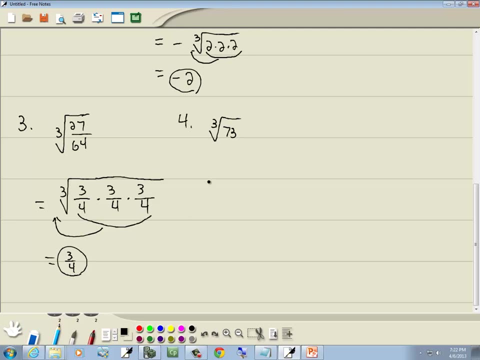 and you want to choose the cube root, the number four, so you can down arrow to it, highlight it and press enter. or you can just press the number four and it'll down arrow and enter for you and that'll put in seventy three and then enter and uh, so this is going to equal to four, point uh. 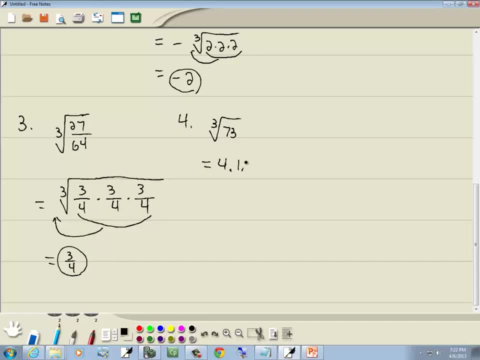 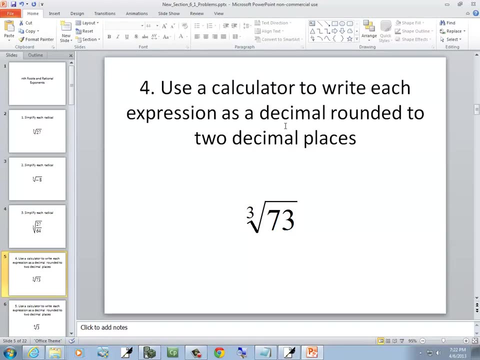 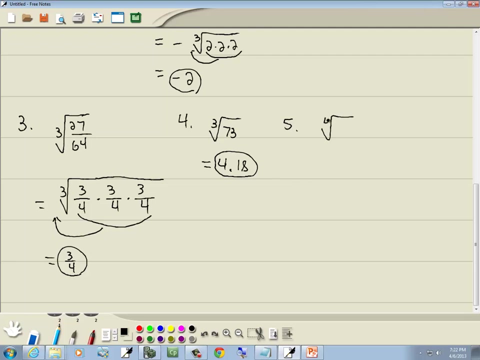 two decimal places. so four point one eight, and that's our answer. okay, next one is a calculator bases. one also forgot four through it, uh three and uh rounded uh two decimal places, again uh three's prime. so we can't andню the prime factorization of it. 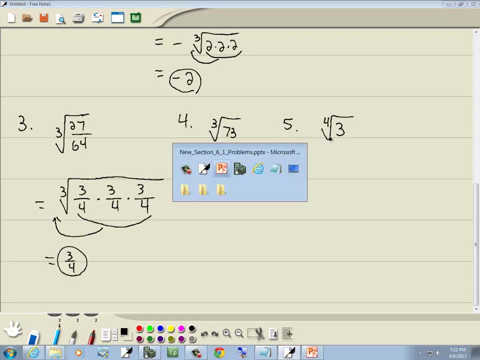 I, that's a broke down to get. so I think we can dalaug in akaka for me taking further than that. uh, three sprims, so we cant do the prime factorization of it. uh, that's as brokedante we cant do is plug in our calculator. if it wants to take it any further, then TO stukin any further than that. 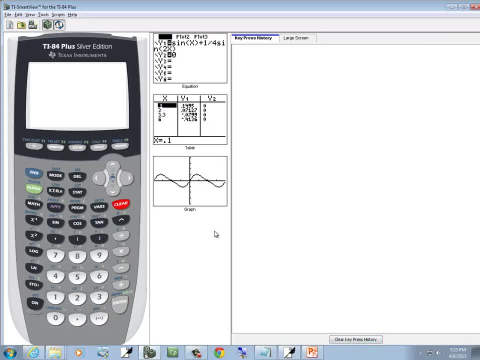 strange on your calculator, to put this one in, you have to put your index in first. so put four in now, choose math, and then I'm gonna choose this fifth one, the one at the radical symbol with an X before it, and if you're got a ta3, ta4 earlier, ta force, you have to put a beginning parentheses. 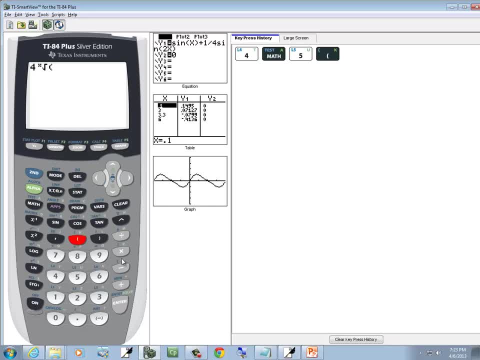 now the newer t84s, you don't have to. it puts it in the radical form for you. it's kind of cool, how does it? and then we'll put three in and then closing parentheses in there. now, if you go ahead and just put three there, it'll work for this problem, but if you have anything more than a, 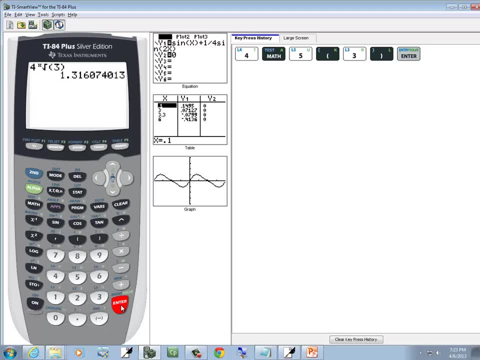 single number there, it won't work. so you should get in the habit of, whenever you put in like a fourth root, fifth root, sixth root or whatever, that you always put a beginning parentheses, and this gives you a little bit of a hint to what the problem is. so I'm gonna go ahead and 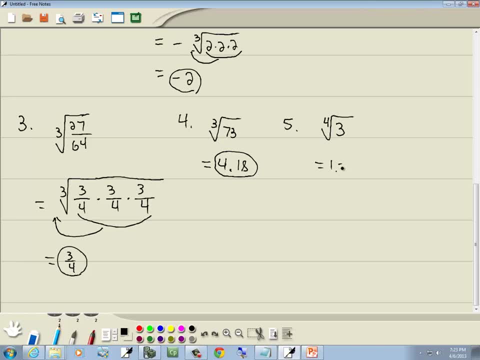 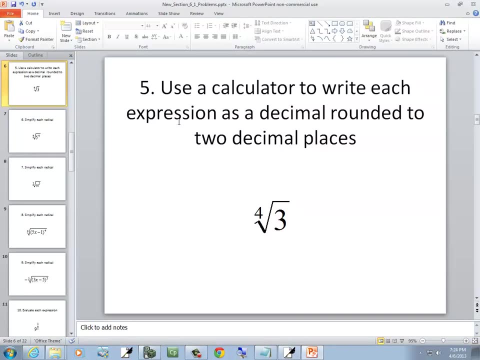 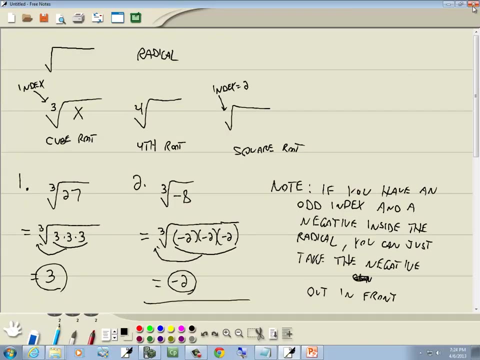 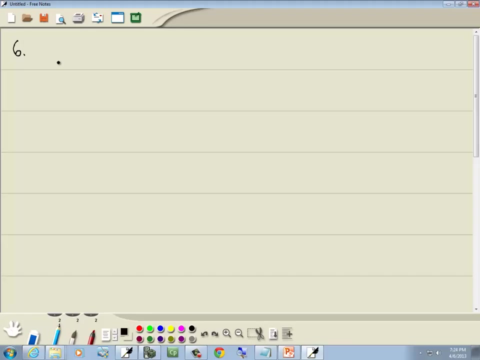 give this one point three, two, and that's our answer. let me start a new page and we'll look at this next one. okay, so we got the fourth root of five to the fourth. well, think what five to the fourth means. five to the fourth means five times, five times five. 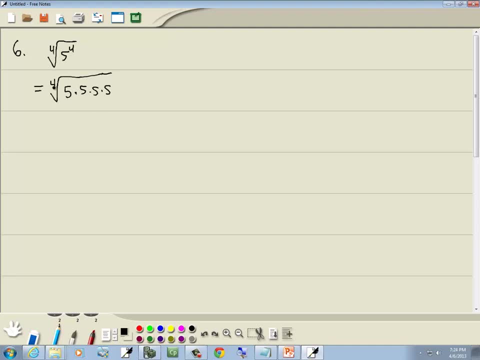 times five. we've got four fives. our index is four, which means we're looking for four of something. well, here's four or five. so those four fives are going to come out in front as a single five, and that's our answer. now it there. 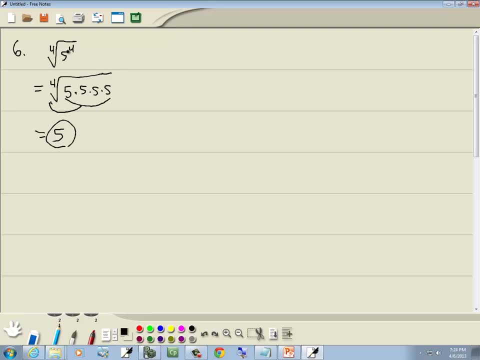 it doesn't work all the time. there's some, uh, special cases we'll need to take a look at, but if your index matches the power, then they basically cancel each other out. you're just left with the whatever. whatever is inside here, like the five. so since this was index of four, this is power four, then automatically. 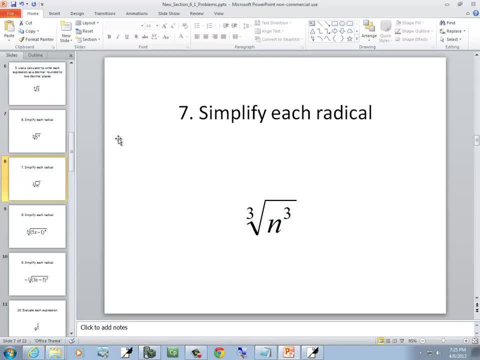 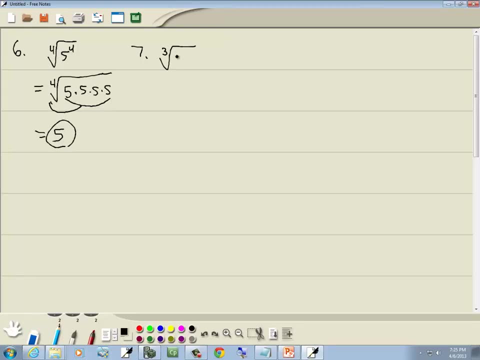 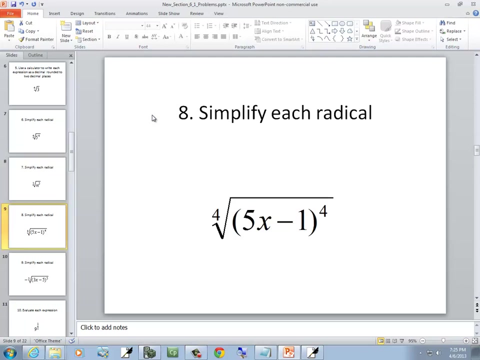 a new answer is gonna be five and, like I say, there's some special cases we're going to talk about. but let's look at this one. our index is three, our power is three, so again, those basically cancel each other way and our answer is in. now, this one here, this is one of our special cases. 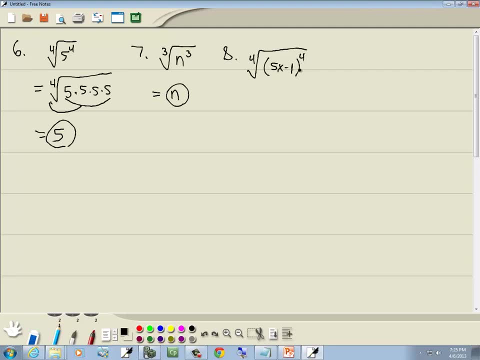 and they understand the answer. you get off of this. first off, let's apply what we've been saying: index is four, our power is four, so basically, those cancel and we're left with 5x minus one. now, if you remember from elementary algebra, algebra one, we'd have items like this: square root of 16. and we'd write that as four times four. 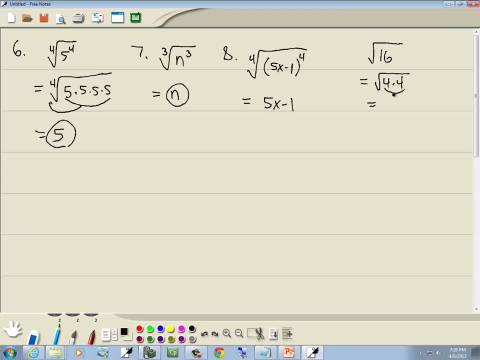 and since this is a square root, we're looking for a pair of somethings. here's a pair of four, so they come out as a single four, but we could also have rewrote this: square root of 16 is equal to negative four times negative four. 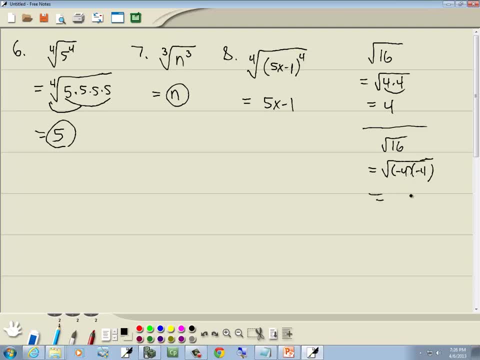 and remember the square root. we're looking for a pair of somethings. well, here's a pair of negative fours, so those come out as a negative four. but in elementary algebra- algebra one- we learned this was actually our answer. this was not our answer, and there's a note that goes along with this. 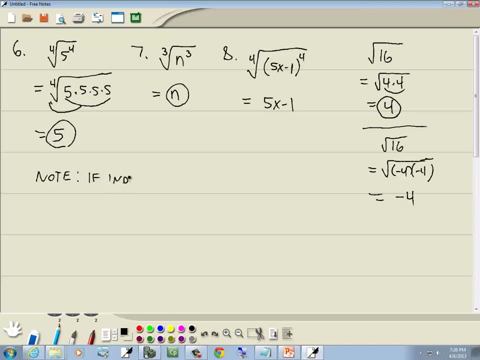 it says: if your index is even, you can only have positive numbers come out. so, if your index is even, you can only have positive numbers come out. that's why our answer here is four, not negative four. well, how's that deal with this problem? well, our index is even. 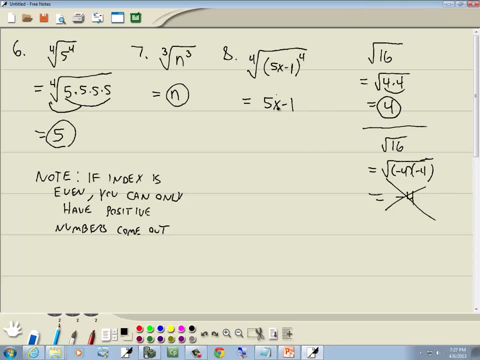 which this says you can only have positive numbers come out. but we have a variable. we actually don't know um what this is. if I put in, X is equal to seven, for example, five times seven is 35. 35 minus one is 34. it's positive. so we're fine. but if I put negative two in for the X, five times negative two is negative. 10 minus one gives 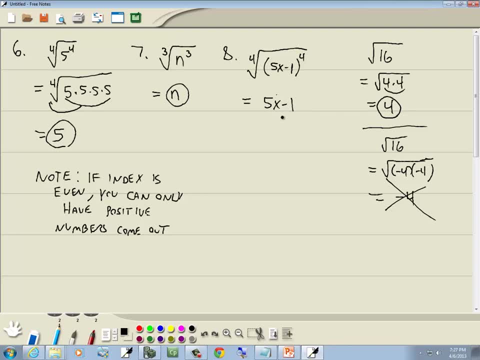 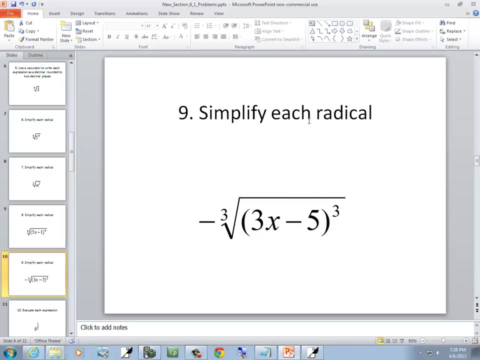 a negative 11 and we can't have a negative number come out of radical with an even index. so how we handle that to make sure it's positive is we put absolute value. bars are on it like that and that's our answer. now, that only applies to even indexes. doesn't apply when you have an odd index. so let's. 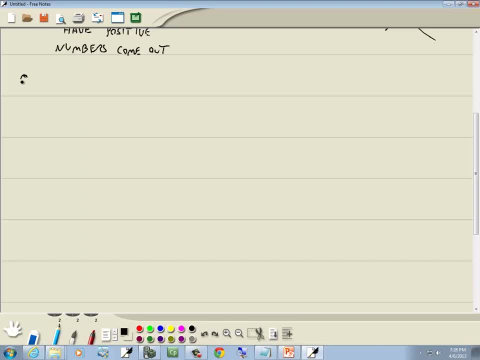 look at this next problem. we have negative cube root 3x minus 5 to the third power. well, this negative, it's out in front, that's just that's out in front. it doesn't change anything, it just stays out in front. now here our index matches the power, so they're gonna cancel each other out and we're 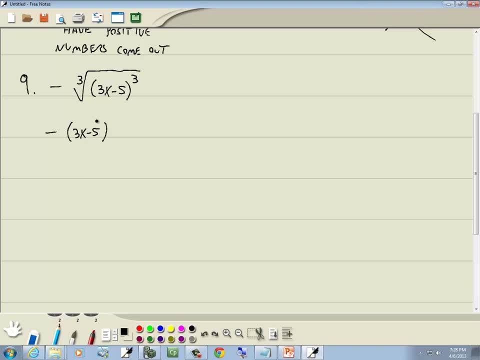 gonna be left with 3x minus 5. now put parentheses around this because the negative that's out in front has to flip the sign of everything now. I didn't worry about putting absolute value bars around this because this was an odd index the only time. 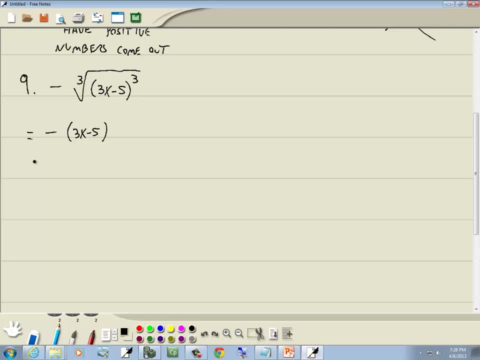 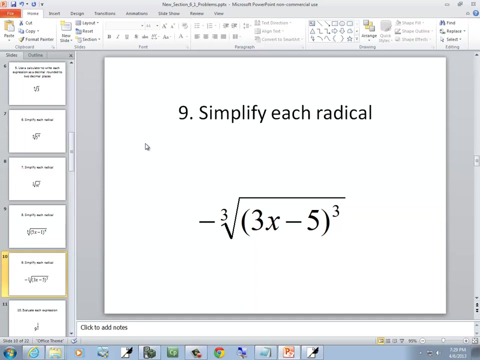 you have to worry about. that is when it's an even index and that negative. we can now take through negative 3x and then plus 5, and that's our answer. now these next ones are going to demonstrate rational exponents. now I like to do this by example. it makes more sense. so we've got 9 to the 1 half power and it says: evaluate each. 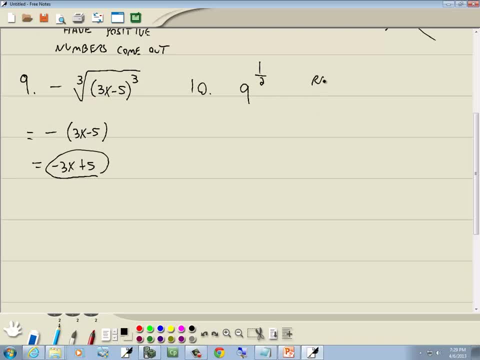 expression. well, this is a rational exponent. not a lot of people don't remember that term and what it means and so forth. so in class a lot of times I say: fractional power form means you're exponent is a fraction. now, to simplify this without using calculator, we need to 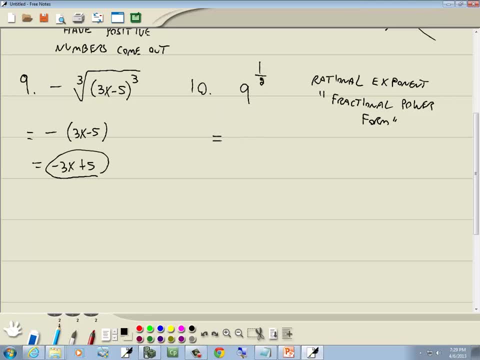 put it back in the radical form. when you see a fractional power like that, that's a radical is just written a different form. so what we're going to do is we're going to rewrite this in this manner: studio now, whatever your denominator is up here, this 2, that'll go in this slot where you're in this small space, and so on. this one is: 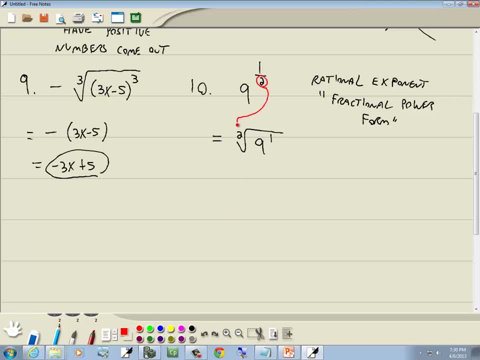 going to work in most other experiences, but it's important that all of this is true and that's the key to this formula tool: to get an idea of good, but by index. that's your index. whatever numbers up on top, this will be your power. so you 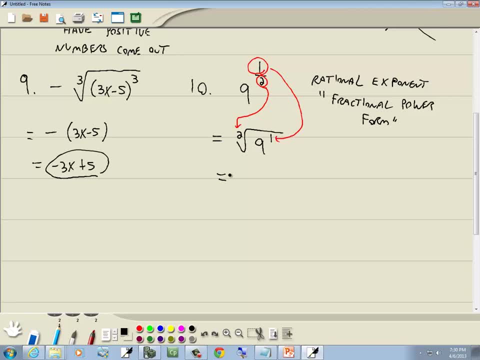 can put it right there. well, whenever our index is 2, we never actually write it. so this is just a square root, and 9 to the first power is 9, now 9. if I do, the prime factorization is 3 times 3. there is no number in a slot here, it's by default 2. 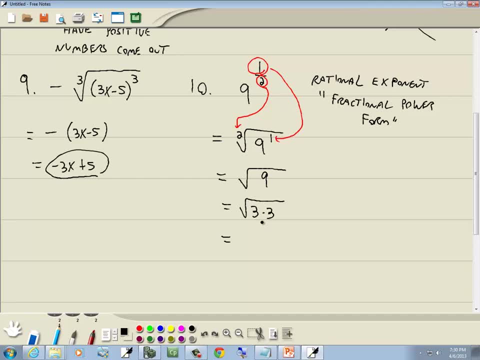 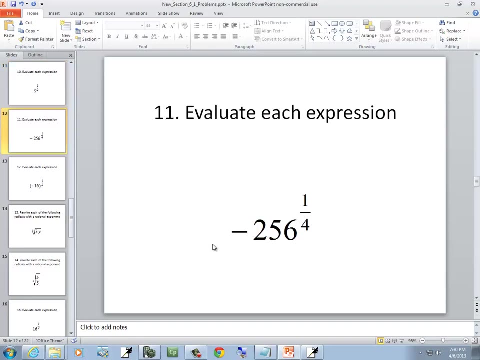 so our index is 2, so means we're looking for a pair of something's 2 of something. well, here's two threes, so those two threes gonna come out in front as a single 3, and that's our answer. this next one has a little note that goes along with it. 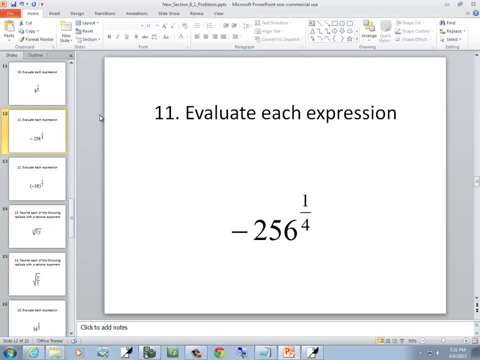 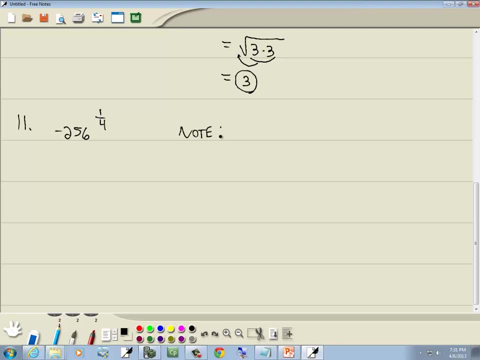 some of these are just to refresh your memory. on exponents, and you saw this note back in elementary algebra 1, it says: a an exponent only affects what is to it's immediate left. so an exponent only affects what's to its to its immediate left. unless there's parentheses, then it affects everything inside of parentheses. 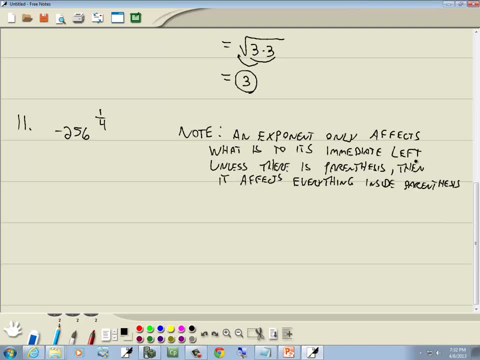 So this one-fourth power you see here only affects the 256. It doesn't affect the negative. So we're going to write this back in the radical form. So this is going to be 256 to the first power. Again, whatever your denominator is the 4, that's your index. 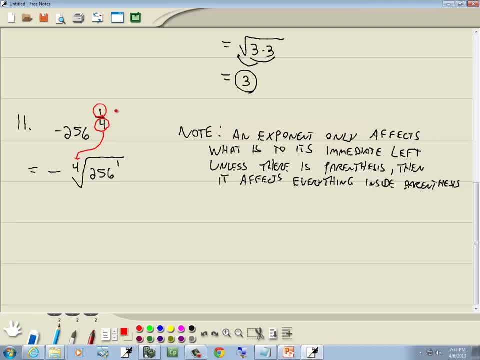 So that goes right there. And whatever number's up on top here, that's your power. That goes right there. Take my glasses off, They're kind of hurting my ears. There we go, Negative stays out in front, and then we've got the fourth root and we want to write prime factorization of this. 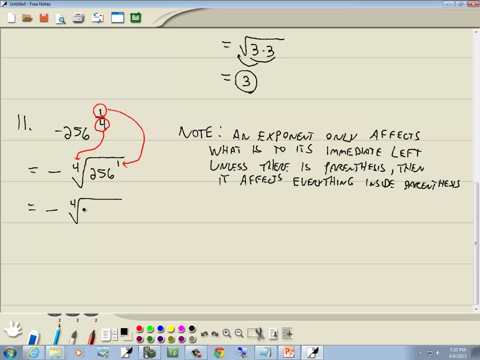 Now we could do the prime factorization, which is a bunch of twos, but this is also 4 times 4,, which is 16, times another 4, which is 16, times another 4, which is 256.. 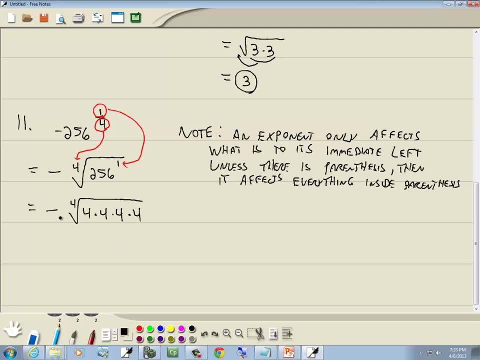 Now our index is 4, so we're looking for a set of 4 of something. Well, here's four 4s, so they're going to come out as a single 4.. And the negative's already out in front, so our answer would be negative 4.. 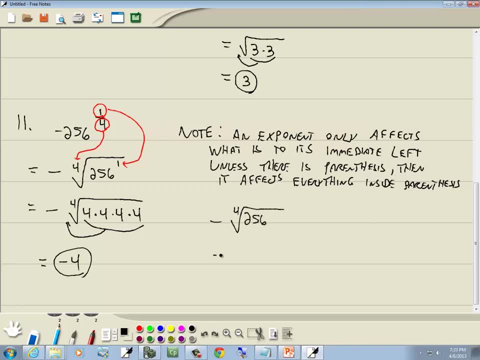 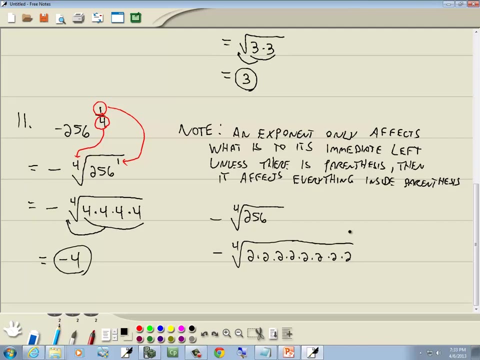 Let me show if you actually did the prime factorization. Prime factorization 256 is eight, twos, two to the eighth power, six, seven, eight. so if we did the prime factorization like that, our index is four. so we're looking for a set of four. 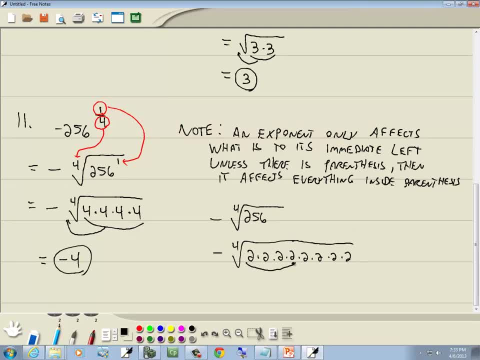 of something. well, here's four twos, so they're going to come out as a single two. well, here's another set of four twos, so they're also going to come out as a single two. try that again. I didn't write that very straight. there we go, so. 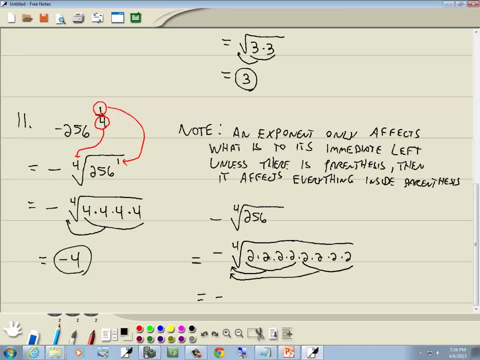 negative stays out in front. this first set of this, first set of twos, this, these four twos, comes out as a single two. and then this set of four set of two's, these four twos come out as a single two and they come out with multiplication. 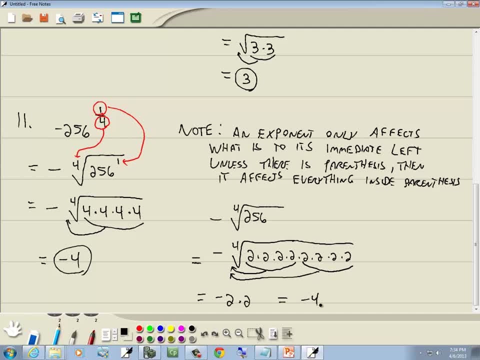 between them. so negative twos times 2 gives us negative 4. so we'd get same answer. so it doesn't matter that if you can't see. it's 4 times 4 times 4 times 4 if you do the prime factorization. 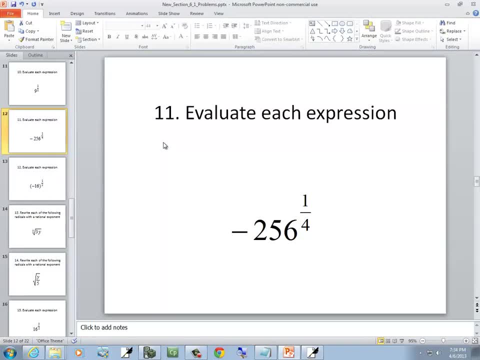 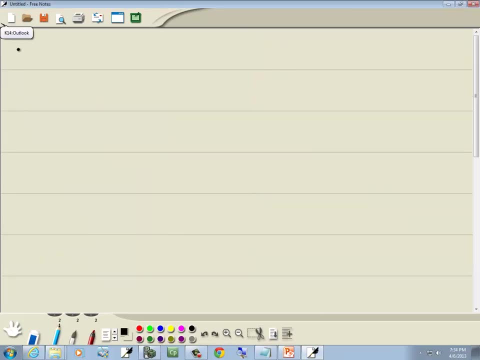 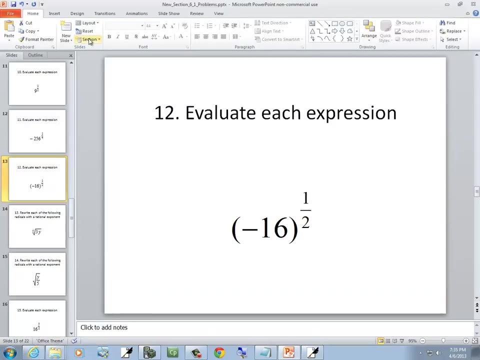 you get the same answer. let's take a look at this next problem, and it has a note to go along with it. by themselves, these problems are fairly simple, but there's a lot, of, a lot of little tricks, a lot of notes that goes along with them. 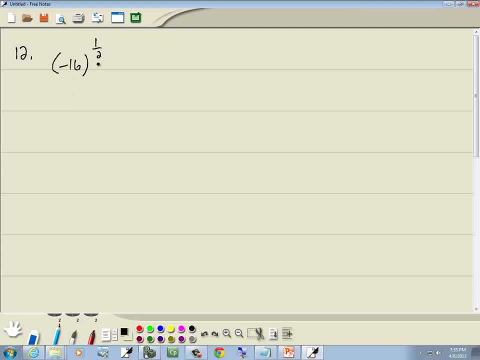 now this one. here, if we look at immediately to the left of our exponent, we have parentheses, so this one-half affects all of this. so when we put this back in a radical form, it's going to look like this again: whatever numbers on the bottom, new denominator is your index and whatever is right here you put right. 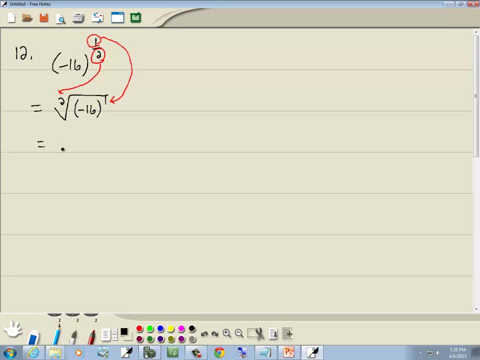 there, which we know, index of two is the square root, so it's become square root and the first power drops away. so we got square root of negative 16. now our note on this: if your index is even and you have a negative number, so you have a negative number. 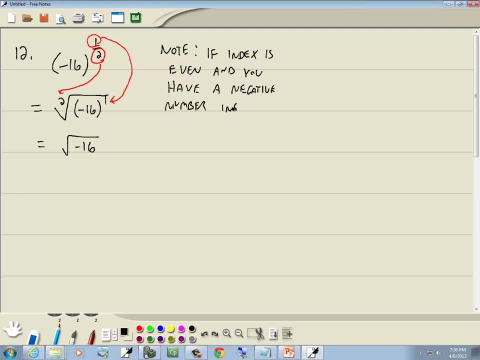 inside the radical, then the answer is not a real number- we actually see later on on different lesson- it's actually an imaginary number. so here, If your index is even here, our index is 2, and you have a negative number inside the radical, Well, we have a negative 16 there. 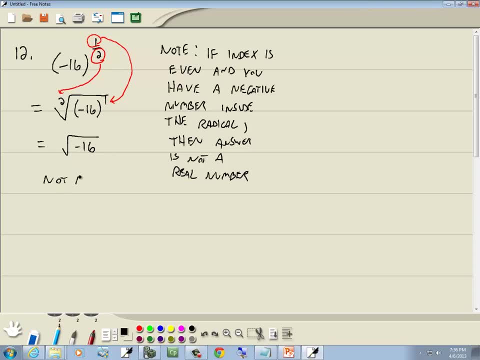 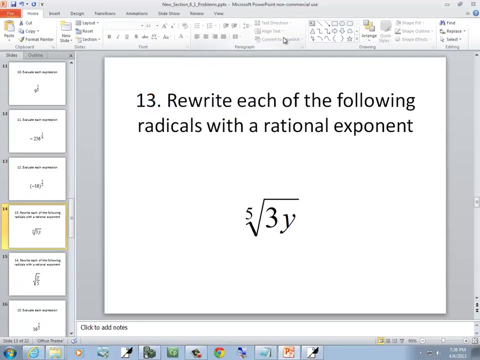 Then your answer is not a real number. So our answer here is not a real number. Let's take a look at this problem. This just kind of builds upon what we've already been talking about. We've got the fifth root. I should write that a little cleaner. 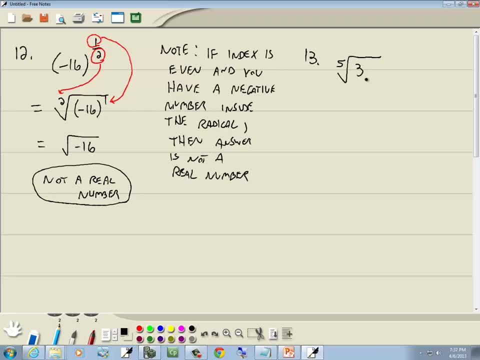 So fifth root of 3y It says: rewrite each of the following radicals with rational exponent: Well, if I were to, If I were to put a power inside, this would become 3y to the first power. So, to go backwards, this would become 3y to the one-fifth power. 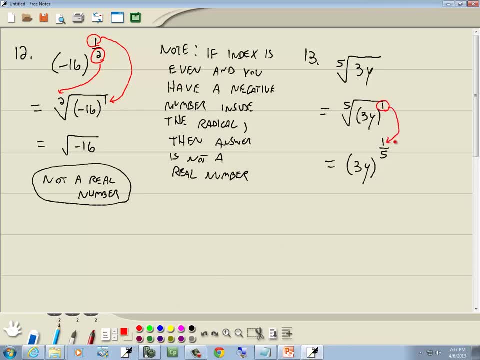 Whatever power is inside here goes up on top, And if you don't have a power- like we just have 3y up here- it's by default 1. You don't even have to write that, And then, whatever our index is, that goes to our denominator. 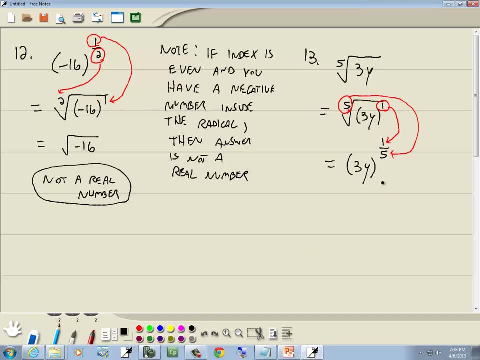 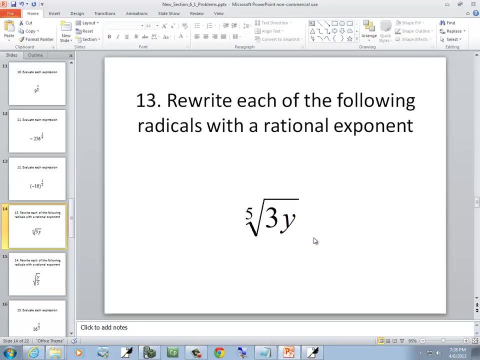 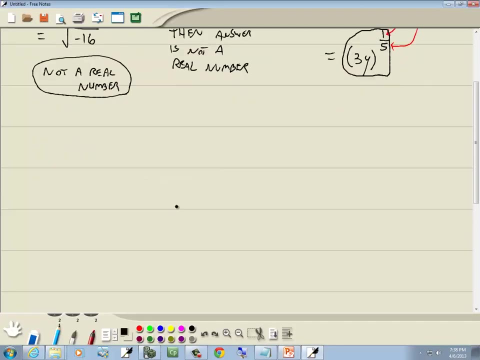 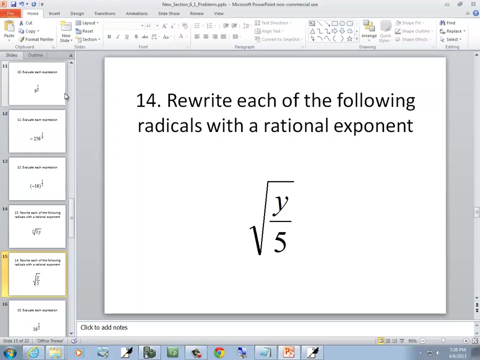 So 3y to the one-fifth power is our answer. Let's take a look at this one, Number 14.. We have the square root of y to the fifth. Well, let's see. Let me put the index in there. 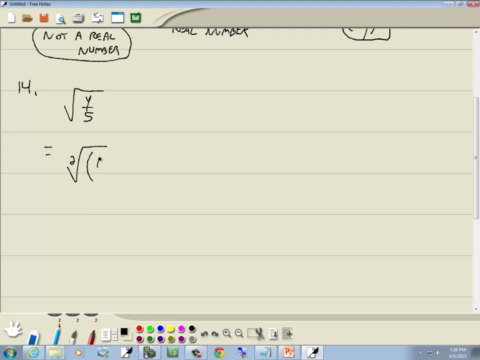 Remember, if you have a square root, it's default 2.. And then again, if I were to put a power here, this would be y to the fifth or y over 5 to the first power. So this becomes y over 5 to the one-half power. 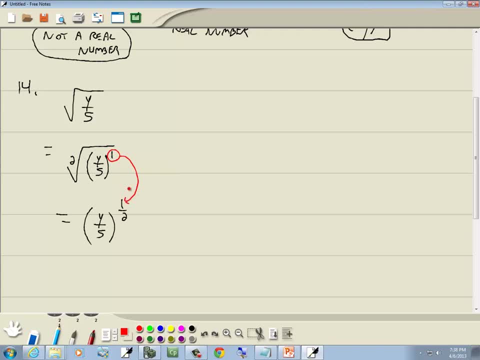 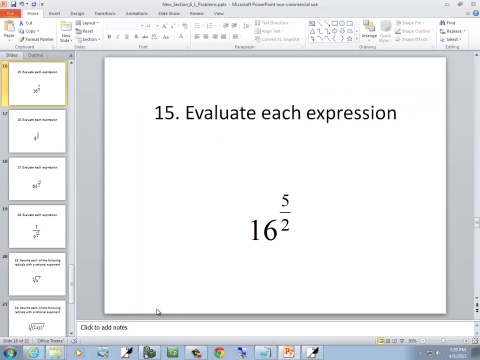 Again, whatever power is here goes up on top And whatever your index is goes down in your denominator. So y over 5 to the one-half power is our answer. And let me start a new page. This next problem is going to take a few steps written down. 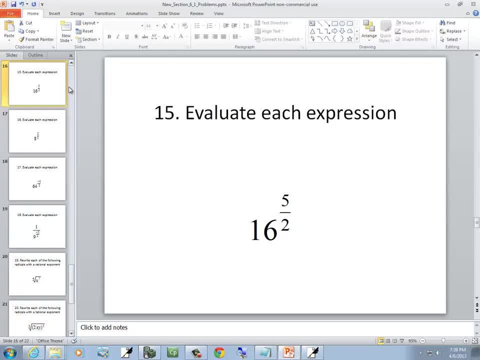 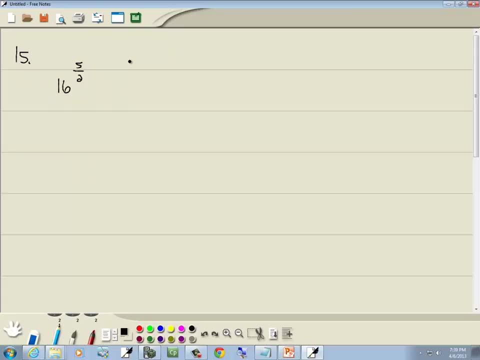 So we've got 15, which is 16, to the five-halfs power, And they want us to evaluate each expression. So this is evaluating A number to a fractional power, rational exponent, So to a fractional power where the numerator, the number up on top, is greater than 1.. 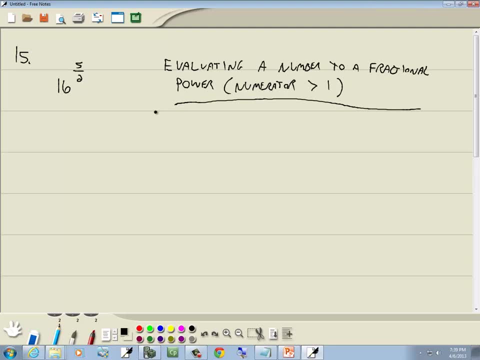 And we've got a property that goes along with this particular problem And I'll write the property down after we work it. The problems are fairly simple. the steps Property makes it look kind of complex, which usually is the case. Our first step is to put the numerator of the exponent. 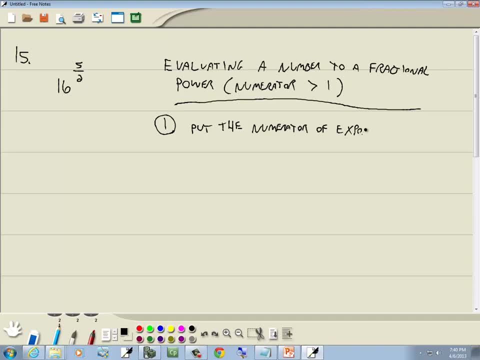 on the outside of a set of parentheses. so this is going to become 16 to the 1 half power raised to the 5th power. now notice, I took the numerator, which is 5, and put it on the outside of the set of parentheses. now where the 5 was in the exponent, I put a 1 step to rewrite what is inside the 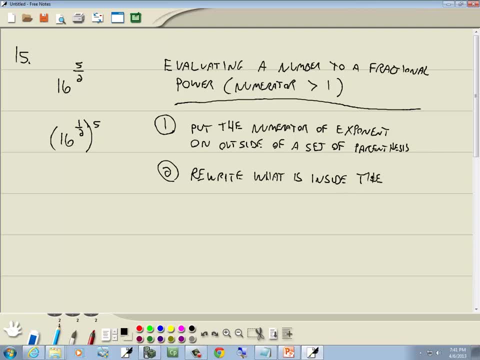 parentheses in radical form and simplify. well, the 16 to the 1 half power, that becomes the square root of 16. 5th power stays there, square root of 16. well, that's 4 times 4 and remember, with the square root our index is 2. so we're looking for a pair of somethings. 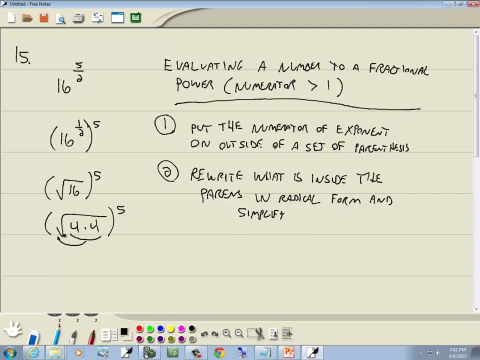 here's a pair of 4's, so a pair of 4's is going to come out in front as a single 4, so we're going to end up with 4 and then the 5th power carries down. now simplify, even not just the radical, but now you. 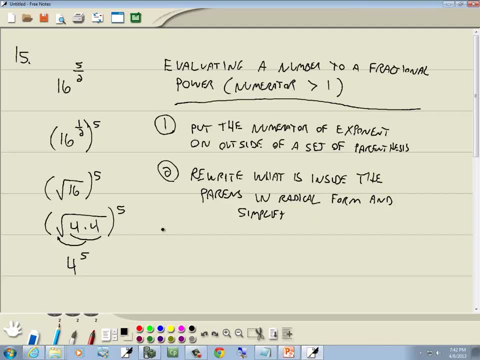 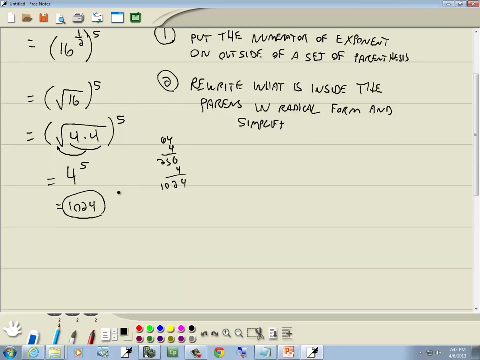 take this: the 5th power, 4 to the 5th power is 1024 and that's your answer. ok, the property for this is something of this form and I'll choose. what variable should I choose? choose m. so if you have m to the a over b power. 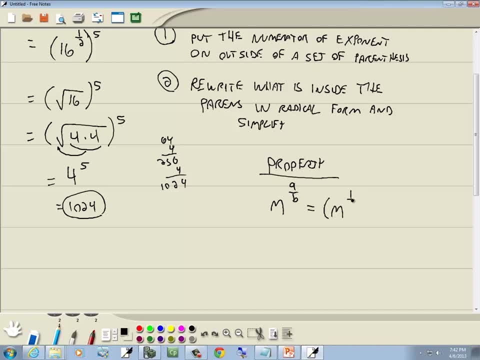 you can rewrite it as m to the 1 over b and you can rewrite it as m to the 1 over b power raised to the a power, or you could rewrite it as m to the a power raised to the 1 over b power. again, that makes it a lot harder than it needs to be. 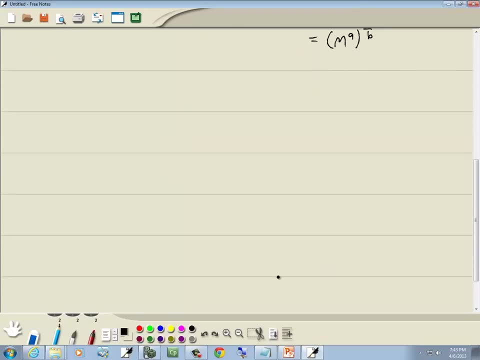 let's take a look at another. one got a to the 2 thirds power. we got a number to a fractional power where the numerator is greater than 1. our first step is again take the number in the numerator of the exponent and put it on the outside sed of parenthesis. so this becomes 8 to the 1 third. 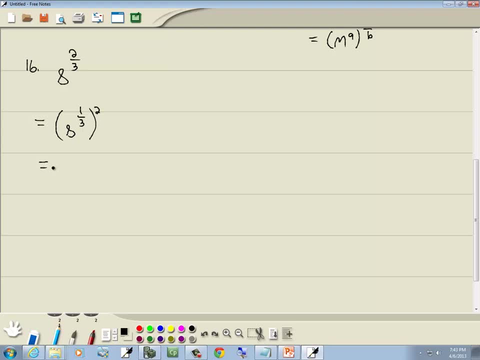 raised to the second power. now, next step is to put this back into radical form, so this becomes the cube root of 8, and simplify- well, if i do, the prime factization of 8. 8 is 2 times 2 times 2.. Now our index is 3, so it means we're looking for a set of 3 of something. 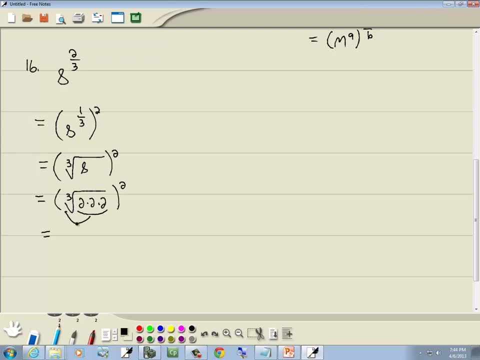 Well, here's 3 2's. So 3 2's are going to come out in front as a single 2.. And then our exponent carries down. So the second power And 2 squared gives us 4.. Let's take a look at number 17.. 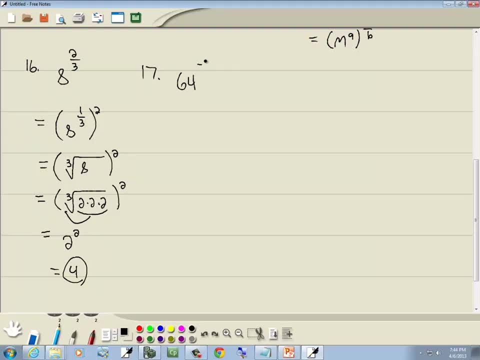 We've got 64 to negative 1 half power And I always like to show this with an example. This is just refreshing your memory, along with some of the techniques in this section, But it's refreshing your memory on how do you handle negative exponents. 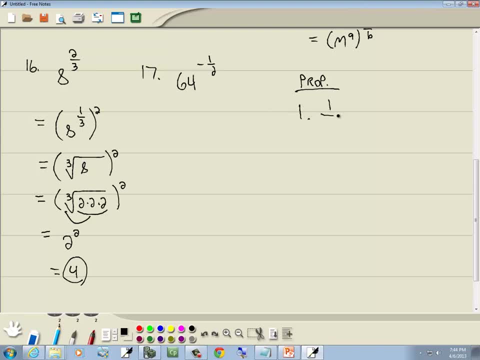 Well, remember, if we have a negative exponent, like we've got 5 to the negative 2 down in the denominator, what you do is you move it opposite where it's at in a fraction. So I take that 5 to the negative 2,. 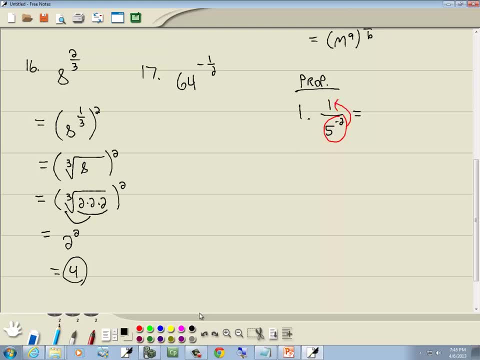 and I take it up on top, Take it to the numerator And it would become 5 to the positive 2.. When you move anything opposite, where it's at in a fraction, the sign of the exponent changes. Now, if we start out with something like this, 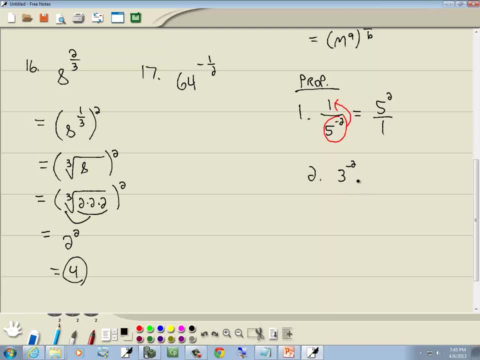 3 to the negative 2,. in order to move it opposite, where it's at in a fraction, you have to put it into fraction. So this would become 3 to the negative, 2 over 1.. And again we're going to move the part with the negative exponent. 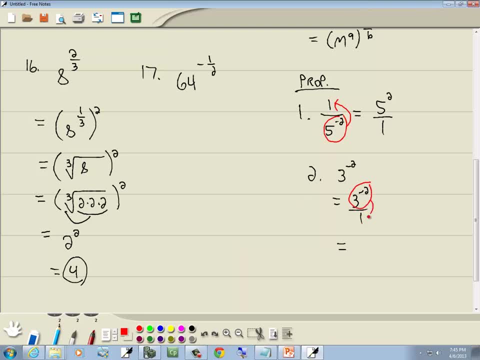 opposite, where it's at in a fraction. So we'll take 3 to the negative, 2 downstairs to the denominator and it becomes 3 to the positive 2.. Well, that's what we're going to do here. We've got a negative exponent. 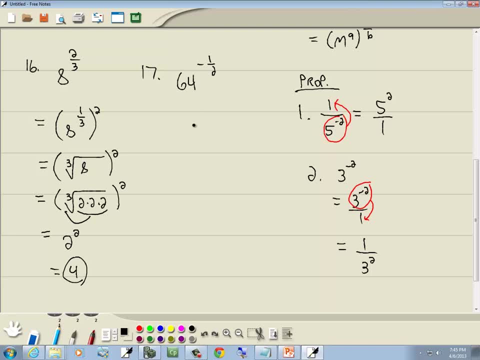 and we want to move it opposite, where it's at in a fraction. Well, it's not in fraction form, so we want to put it over 1.. And now I want to move the part with the negative exponent, the 64, to the negative 1 half. 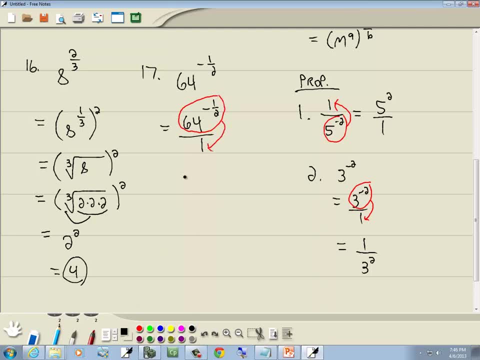 opposite, where it's at in a fraction. So I'll take it downstairs and it'll become 1 over 64 to the positive 1 half. Now we want to put that back into radical form: 64 to the 1 half is the square root of 64.. 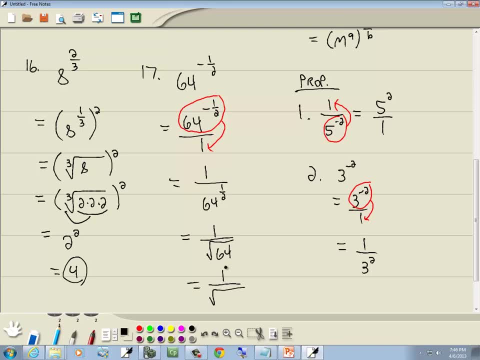 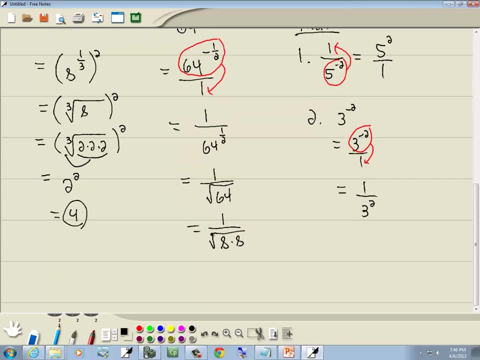 And square root. we're looking for a pair of somethings: 64 to the 1 half is the square root of 64. And 64, we can rewrite as 8 times 8.. So our index is 2.. 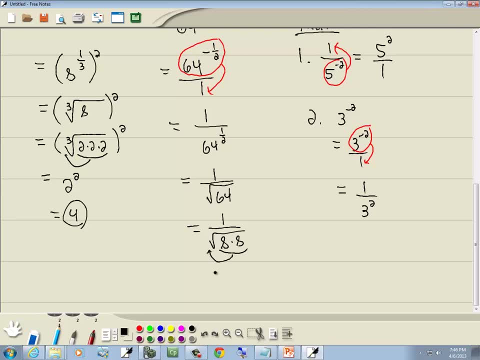 It's a square root. So we've got a pair of 8.. So a pair of 8 is going to come out in front as a single 8.. So our answer is 1- 8.. Let me start a new page. 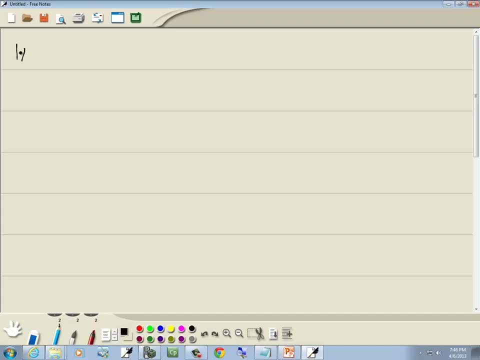 And let's look at this next one. We've got 1 over 9 to the go away. I've asked 1 over 9 to the negative 3 halves Again, we never want negative exponents, So I'm going to take that 9 to the negative 3 halves. 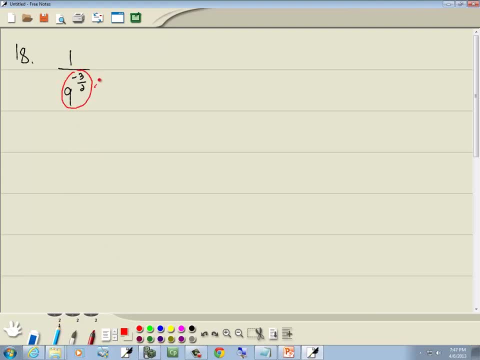 and move it to the top. And again, when you move anything opposite, where it's at in a fraction, the sign of the exponent changes. So it becomes 9 to the 3 halves over 1.. Of course that 1 can disappear. 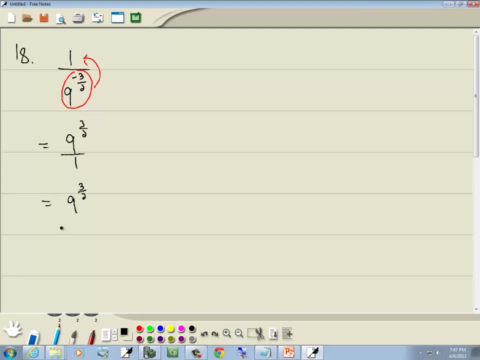 So we've got 9 to the 3. 9 to the 3 halves. Well, now we have a number to a fractional power where our numerator is greater than 1.. So we're going to use those two steps. We're going to take the number in the numerator. 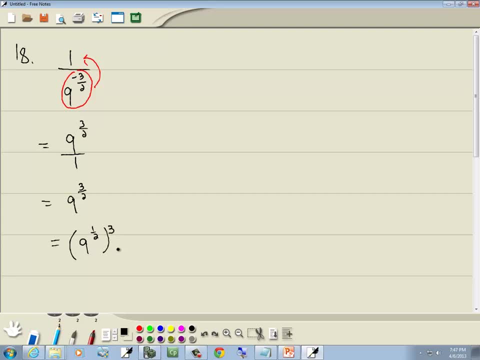 put it on the outside of the set of parentheses. Then we want to rewrite what's inside the parentheses in radical form. So 9 to the 1 half is the square root of 9.. And then the third power carries along And simplify. 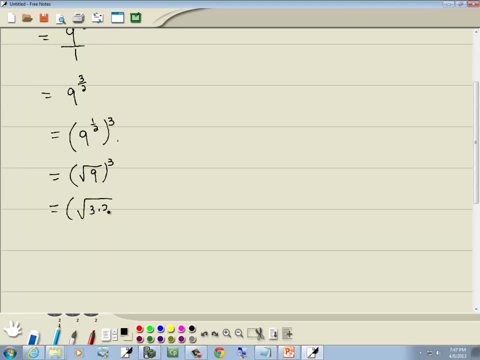 Well, 9 is 3 times 3.. Our index is 2 because it's a square root. So we're looking for a pair of somethings. So here's a pair of 3s. So a pair of 3s is going to come out in front as a single 3.. 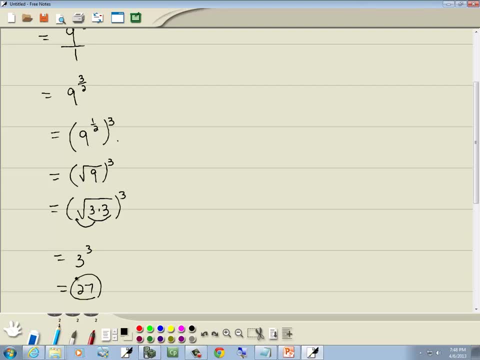 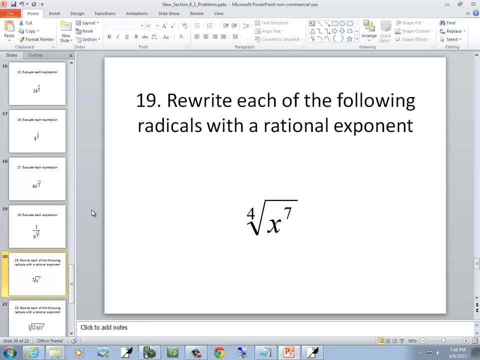 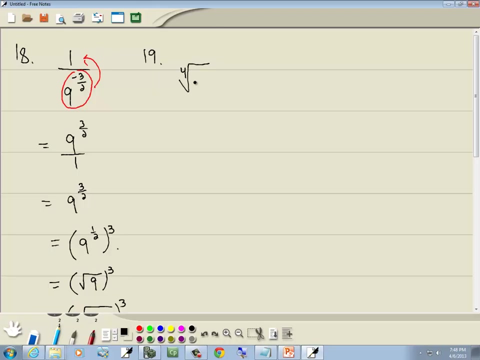 And then 3 to the 3rd gives us 27.. And that's our answer. Okay, On this one we've got the 4th root of x to the 7th, And here's just a few more. Rewrite them in rational exponent form. 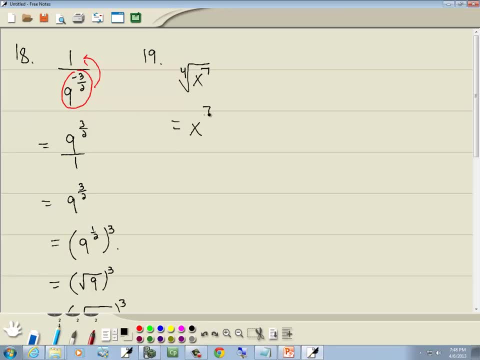 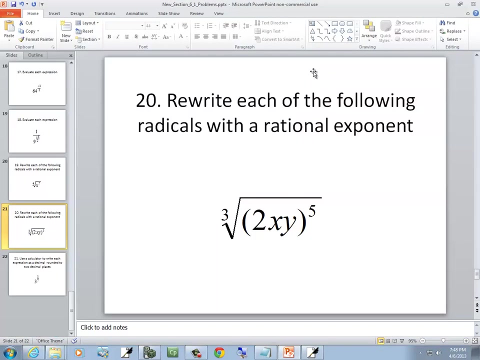 So this is going to become x to the 7th 4th power. Again, whatever power is here goes up on top, And whatever your index is goes in your denominator. So that's our answer. And then we've got the cube root of 2xy to the 5th power. 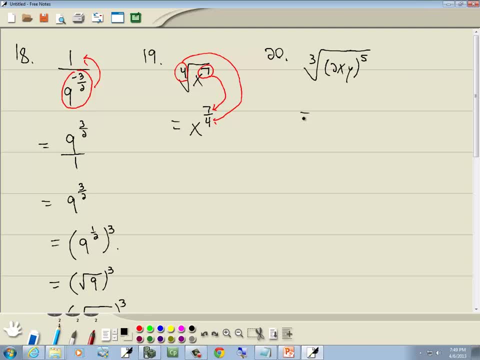 And again, we're going to put this in rational exponent form, fractional power form. So this will become 2xy to the 5 3rds power. And that's our answer. And last problem, it's a calculator one. 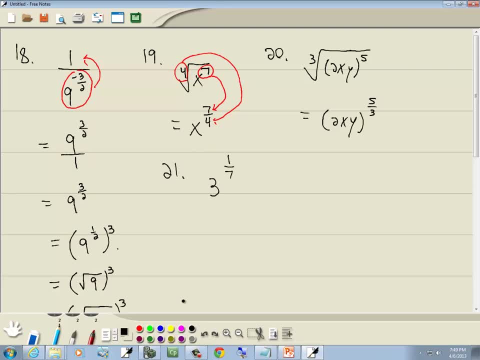